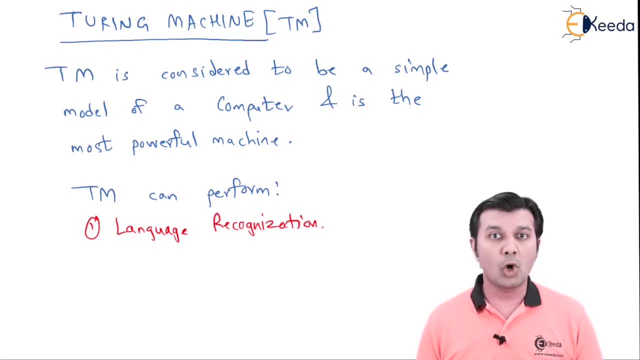 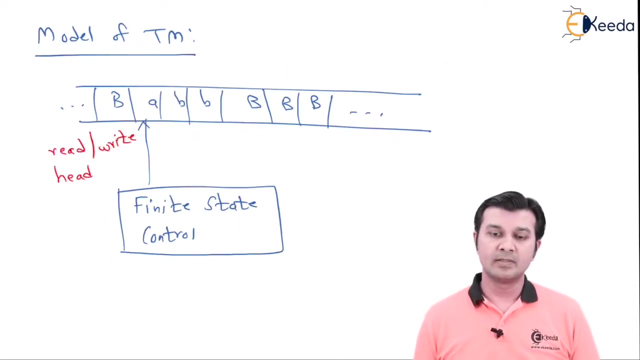 automata's non-deterministic case, without being non-deterministic in nature, then it can also perform evaluation of some functions going ahead. next we have the model of the Turing machine. now, friends, if you look at the model over here, I see over here a tape and this tape. 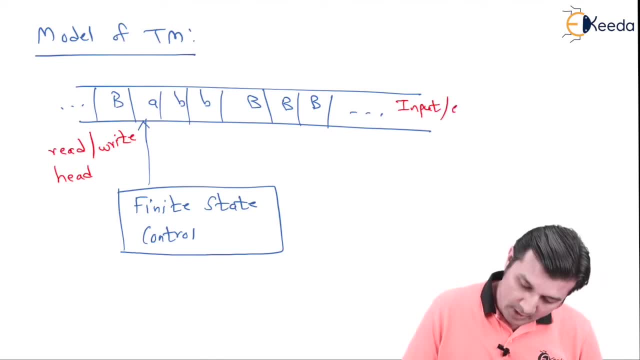 over here is called as not only the input tape, but it is also called as the input slash- output tape. the reason is: on the same tape I can have my input, which I can get converted to the output. also, due to this possible capability, I can now perform addition of the two numbers and show the result on the same tape. or 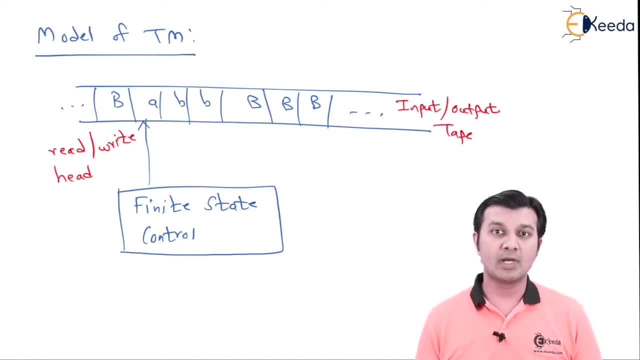 any such kind of mathematical computation and show the answer on the same day. so that is the power of this particular machine. so I have a input output tape. I do have a finite state control and finite state control is going to be the brain of the Turing machine and this brain is going to work. 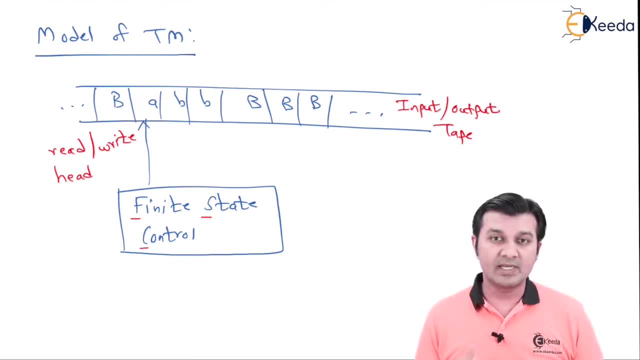 on the input output tape, and it can either change the contents of the input output tape or keep it the same, or it can also move the read head either to the right or to the left, which previously was not the case in the machines that we discussed. 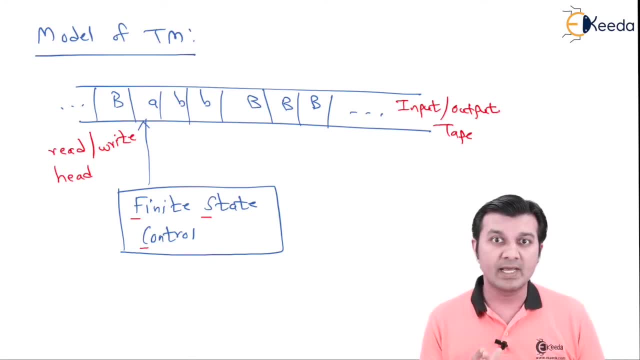 Previous heads were only moving to the right. Now Turing machine's head can either move to the right or to the left, or it can also stay at the same place, right. So we have a read-write head over here, and we do have a finite state control. 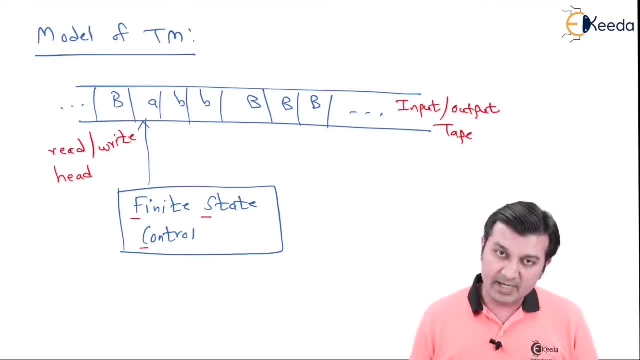 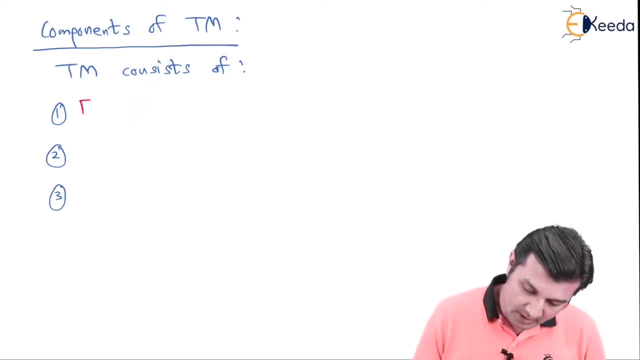 So, going ahead, let me write down the components of the Turing machine now. So we saw that there are essentially three components. The first one is: it is going to have finite set of input slash output states. Next, it is going to have 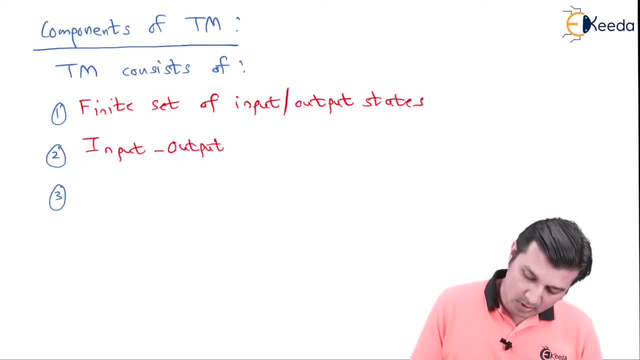 a finite set of input slash output states. Next, it is going to have a finite set of input output tape and it also has a read-write head. So these are the basic three components of the Turing machine to the working of the Turing machine. 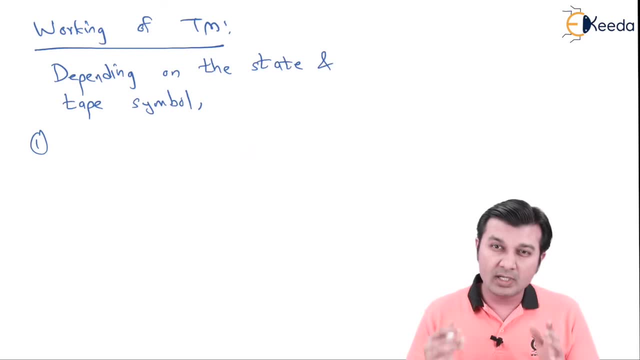 Now in working we are going to say, depending on the current state and the tape symbol- we are not talking of the stack over here- Everything is going to be on the tape. So that is the next advantage of it. We do not require a special data structure to understand the language. 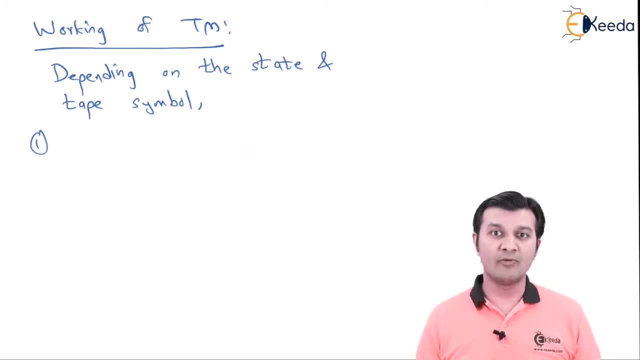 We can do the same thing on the same tape with the help of editing on the tape or manipulations on the tape. Therefore we say, depending on the current state and the tape symbol, my Turing machine can change the state or it can also remain in the same state. 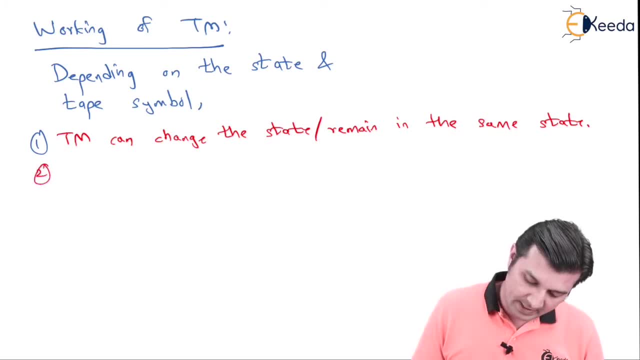 Secondly, I say my Turing machine can change the tape symbol or it can also keep it the same. Third: my Turing machine can move the head either to the left or to the right, or it can keep in the same place too. 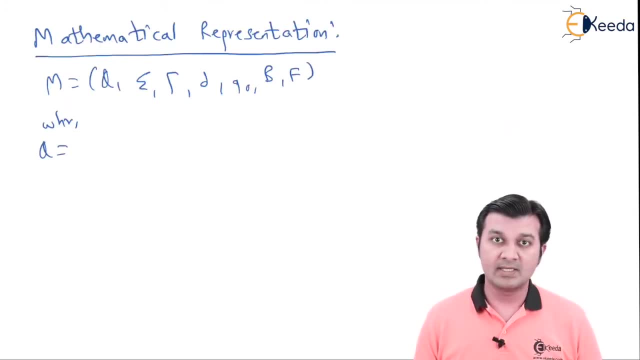 So mathematically a Turing machine is represented as: M is equal to Q, summation G del Q0 BF. Previously it was ZF, Now it is BF. So B over here on the Turing machine stands for a blank symbol. 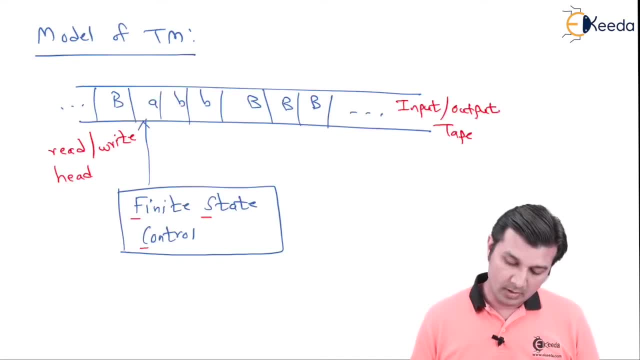 So if you observe this model, in this model we see that the tape has the symbols A, B and B Rest. all of the symbols are capital Vs, And capital Vs in Turing machine are called as my blank symbol. Now, one more interesting aspect of this tape over here is: this is an infinite tape going. 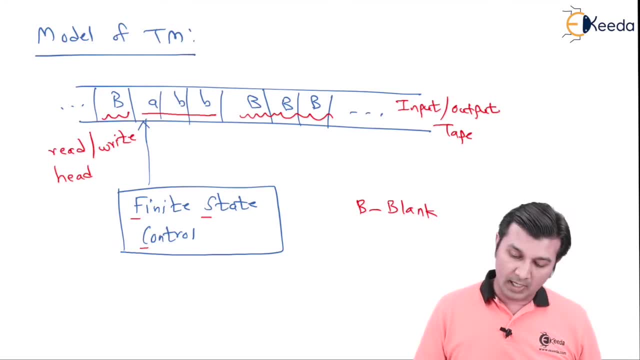 in both the directions. You can see there is a dot dot dot on the right side of the tape as well as on the left side of the tape. That symbolizes that anything which is not shown on that side consists of all the blank. 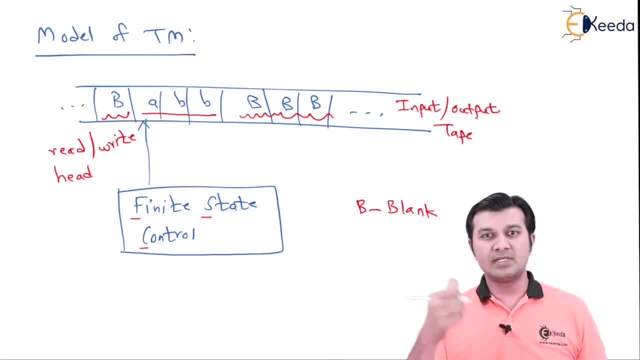 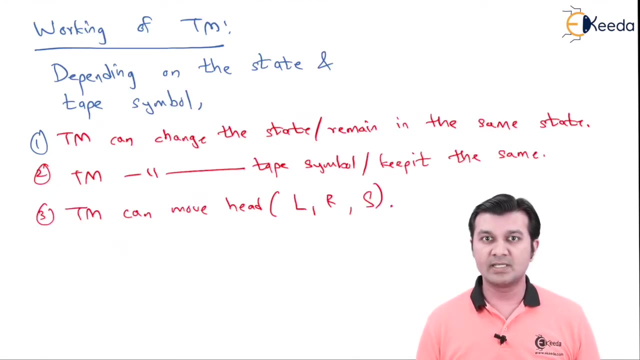 symbols. So previously we used to call this side empty and this side empty as epsilons. Well, now Turing machine gives it a special representation, denoting it by a blank symbol. Okay, So let us go ahead to the representation now. 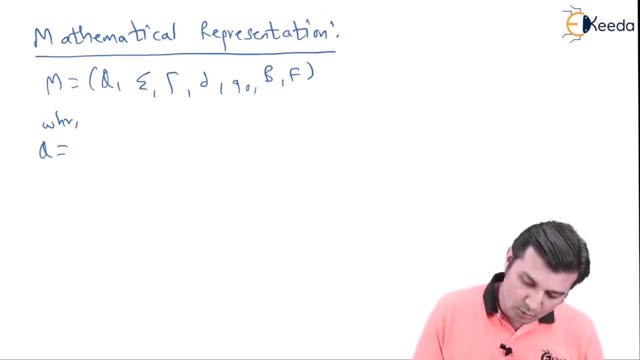 So I say M is equal to Q. summation G del Q0. BF, where Q is going to be my finite set of states, Summation is going to be as usual, my input alpha bed. Del is going to be my transition form. 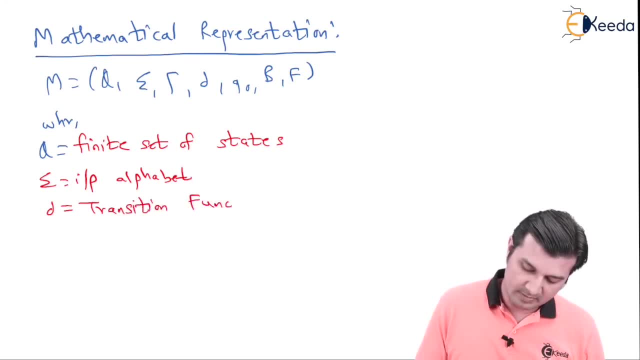 Okay, So this is going to be my transition function, which over here we write as Q cross, G is going to give me Q cross, E cross, either left or right, or do not change the V right head to the left or right. That is the same state. 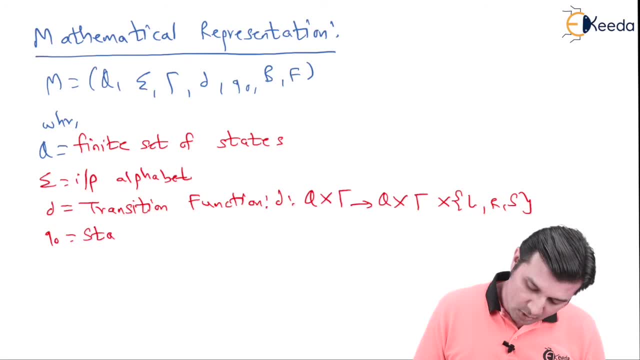 Next we have Q0. Where Q0 is called as Q0. Okay, So Q0 is going to be as the start symbol and Q0 is going to belong to capital Q. Next we have B. As I told you just now, B is the symbol to represent what blank. 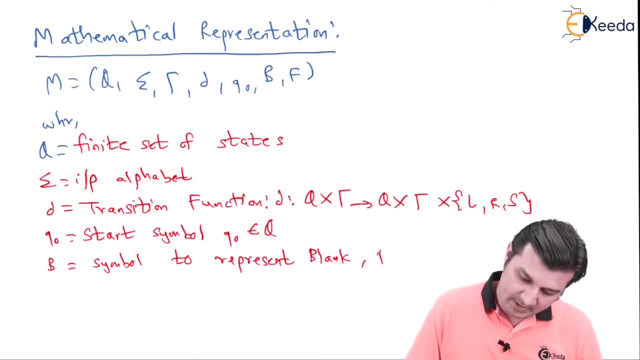 So B is the symbol to represent blank. Okay. So B is the symbol to represent blank, Okay. So this blank is going to belong to T ghi, Next F. Lastly, over here is my finite set of final states, and F is a subset of Q. 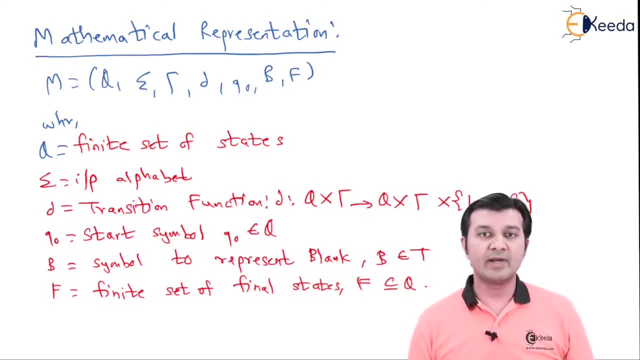 So that is how we define the mathematical representation M-chain. Okay, Thank you, Thank you. m is equal to Q, summation G del Q0, V and F over here. So, having this background of Turing machine, now we can go and try to solve some problem on it. to understand: